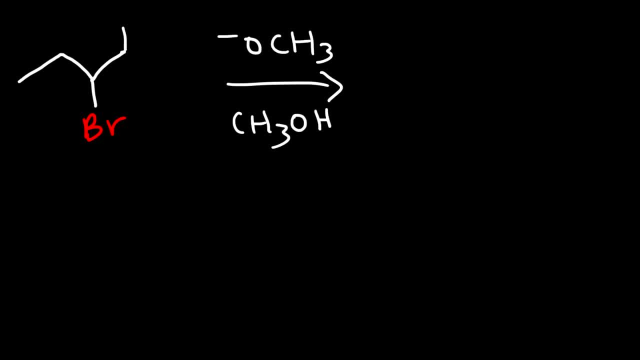 Now the strong base can either go for this hydrogen, the primary blue hydrogen, or it can go for the secondary green hydrogen. Now methoxide can grab both hydrogens. So let's say, if it goes for the blue hydrogen we are going to get a double bond on a primary carbon, The E2 reaction. it's a 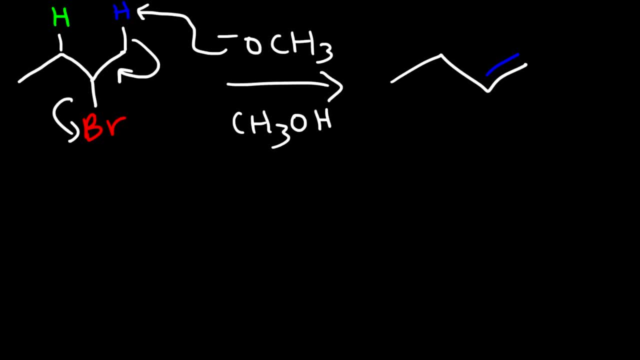 concerted reaction mechanism. It all happens in one step, and so there are no carbocation rearrangements. For the E2 reaction, the rate depends on the concentration of the substrate and the concentration of the hydrogen, So we're going to get a double bond on a primary carbon. 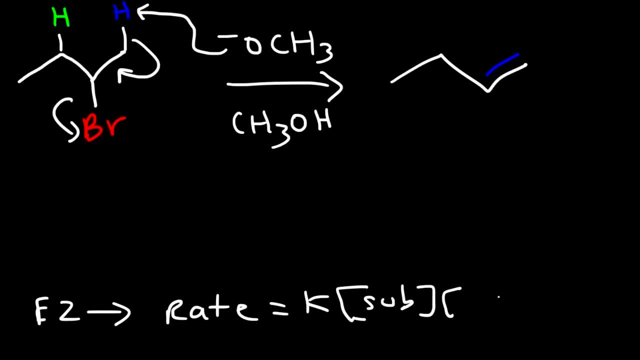 And the concentration of the base. So it's first order with respect to the substrate, first order with respect to the base, but it's second order overall. So if you double the concentration of the substrate and triple the concentration of the base, the rate will increase by a factor of six. 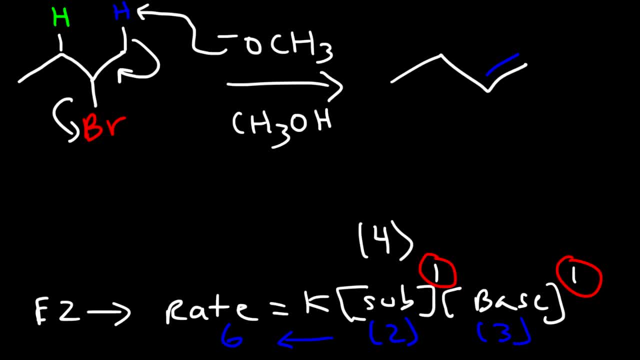 Two times three is six. If you quadruple the concentration of the substrate and increase the concentration of the base by a factor of six, the rate will increase by a factor of six. The rate will increase by a factor of five. The rate will increase by a factor of 20.. 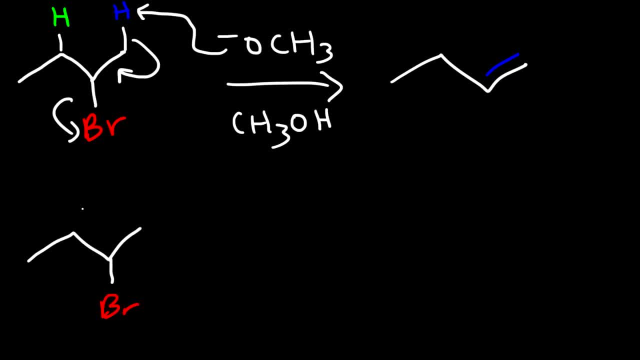 Now, if methoxide goes for the green hydrogen, we're going to get two butene as opposed to one butene. So once it acts as a base grabbing the hydrogen, the carbon-hydrogen bond will break. Those electrons will be used to form the. 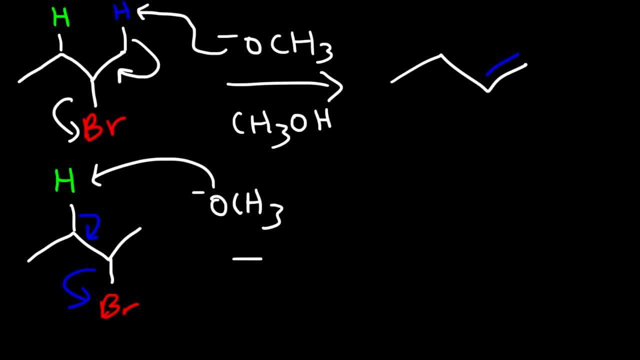 pi-bond, thus expelling the leaving group, and so we can get trans-2-butene. Now there's two green hydrogens here, So one of them will lead to the trans-isomer and the other one will lead to the 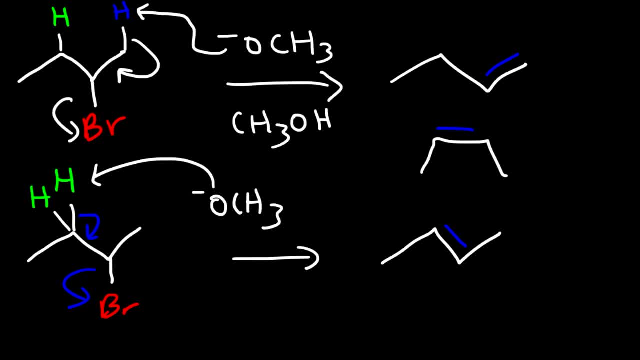 cis-isomer, And so we get a mixture of products. However, we're going to get the zeta product, which is the most stable alkene. Trans-disubstitute alkenes are more stable than cis-disubstitute alkenes. 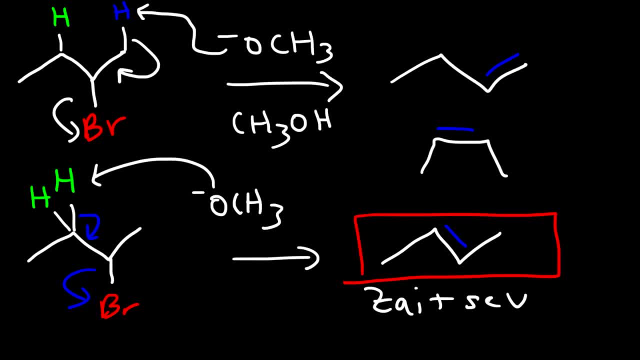 So this one's going to be the major product. This is a monosubstituted alkene. It has one R-group attached to the carbon-carbon double bonds, And this one is a disubstituted alkene. It has two R-groups. A disubstituted alkene is more. 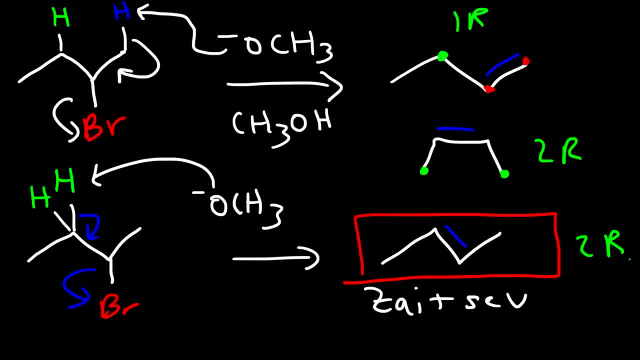 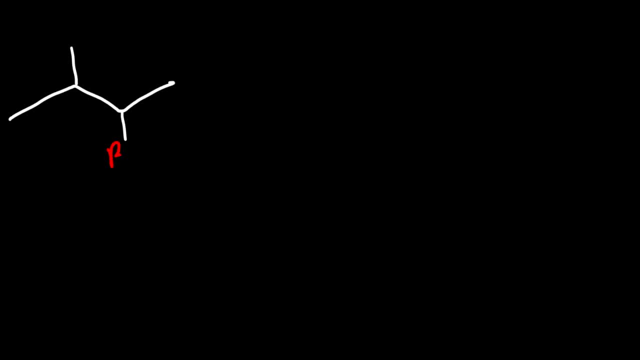 stable than a monosubstituted terminal alkene. Now let's work on some other examples. So here we have a secondary alkyl halide and let's use another structure. So we're going to have a secondary alkyl halide and let's use another. 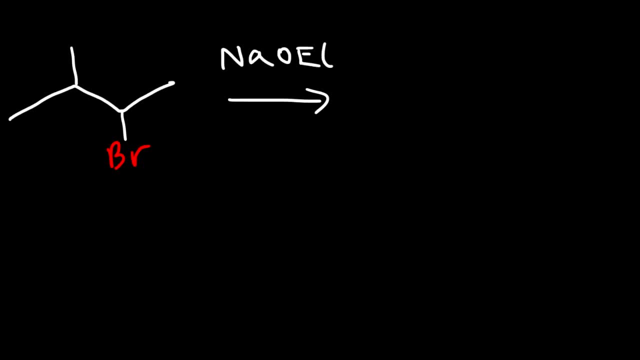 strong base, Sodium ethoxide dissolved in ethanol. Whenever you see ET, ET stands for ethyl, So that's CH3, CH2.. Now, sodium ethoxide: it's going to go for the blue hydrogen as opposed to let's call this the yellow hydrogen, When you use a strong base that is not sterically. 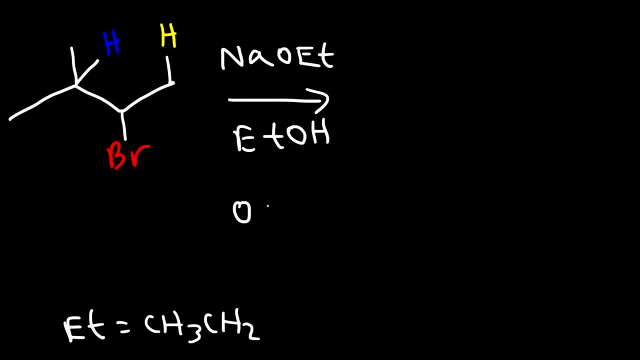 hindered, like ethoxide or methoxide. it's going to go for the hydrogen that leads to the Zasev product. that is, the most stable alkene. So it's going to go for the blue hydrogen forming a carbon-carbon bond. 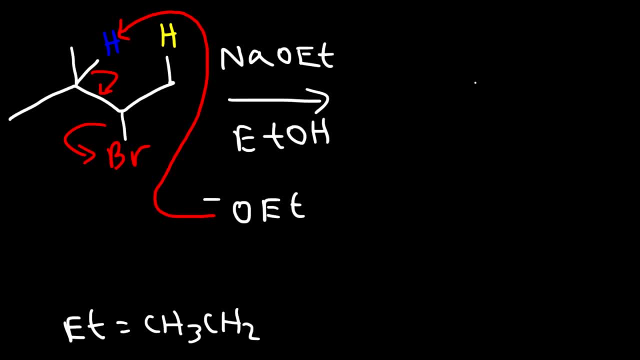 a carbon-carbon double bond, rather kicking out the leaving group, And so this is going to be the major product And this is called the Zasev product. Now, if it goes for the yellow hydrogen, it's going to give us the minor product. 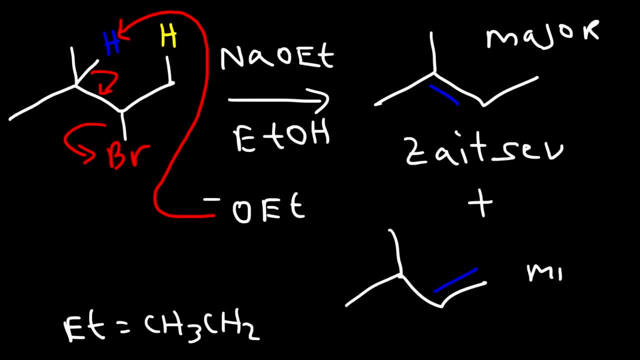 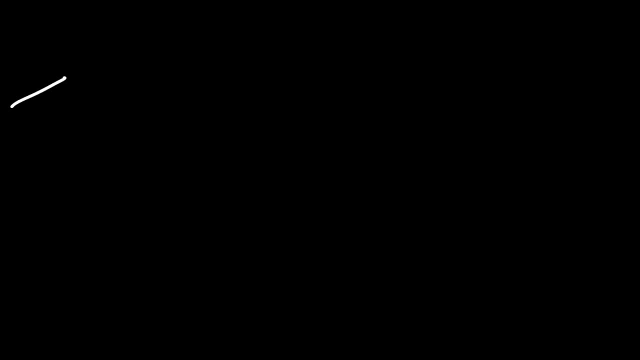 And the minor product is known as the Hoffman product. So this is going to be the major product in this reaction. Now let's look at the Zasev product. Now let's start with the same substrate, In this case 2-bromo-3-methyl-butane. 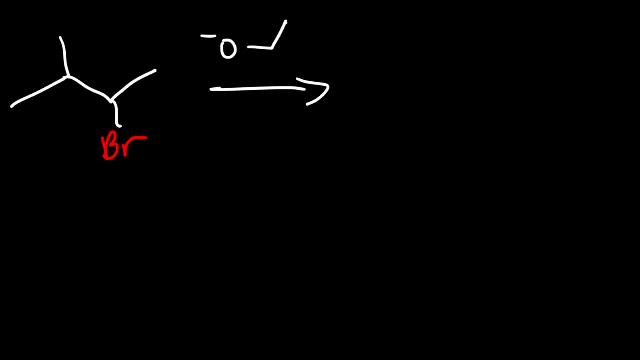 And this time we're going to react it with a bulky base, a base that is sterically hindered Tert-butoxide dissolving tert-butanol. So what's going to happen if we use this base? Is it going to go for the blue hydrogen? 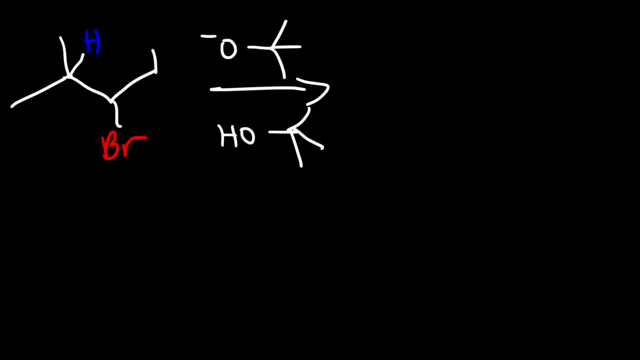 or the Zasev product For the yellow hydrogen. Now, keep in mind, there's three of these yellow hydrogen atoms, But there's only one blue hydrogen atom, Because tert-butoxide is so bulky and because this is a tertiary carbon. 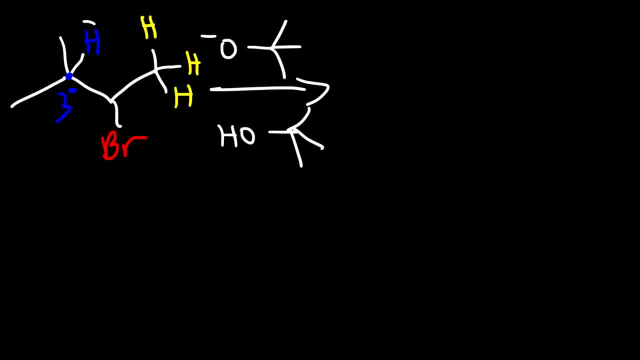 it's going to have a hard time trying to abstract that proton Because it's surrounded by these bulky methyl groups And tert-butoxide itself is also bulky, So it's going to be hard to get that hydrogen that it wants to get. 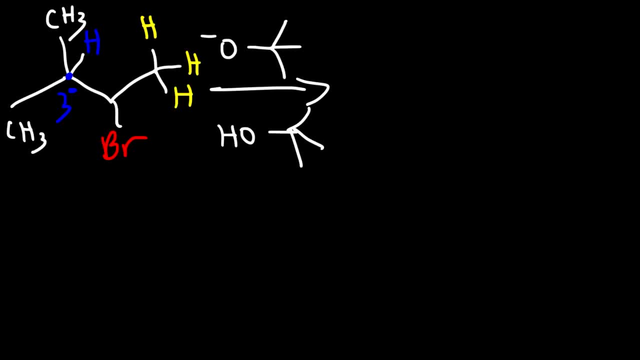 Therefore, due to steric factors, tert-butoxide will prefer to abstract a more accessible proton. In this case, it will preferentially go for the yellow hydrogen as opposed to the blue hydrogen. The yellow hydrogen is on a primary carbon. 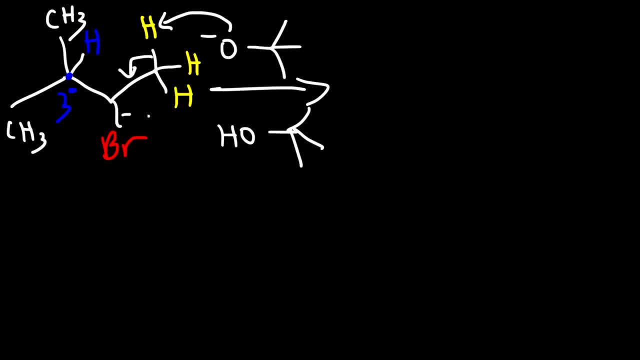 And so it's more accessible than the blue hydrogen. So tert-butoxide will favor the Hoffman product over the Zasev product in this case, if this hydrogen is sterically hindered due to the methyl groups on it. If it's not, then tert-butoxide can go for any of those hydrogens. 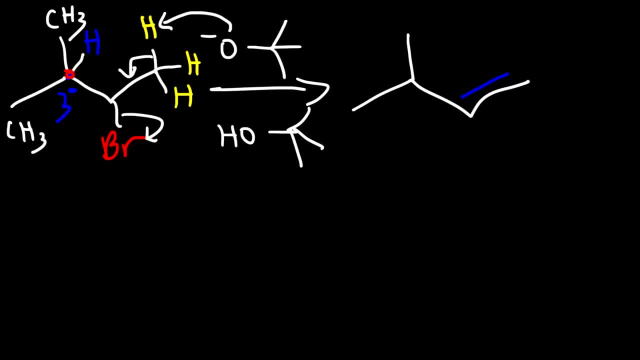 But since the blue hydrogen is basically sterically hindered by the methyl groups, it's going to be hard for it to go there. So this is going to be the major product, In this case the Hoffman product. Now here's a question for you. 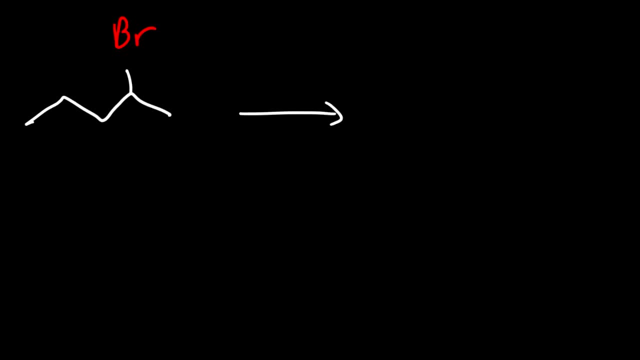 What are the major products for these two reactions? Let's use sodium, methoxide and methanol And also an alkyl fluoride with the same reagents. So draw the major product for each of these two reactions. For the first example, we have an E2 reaction. 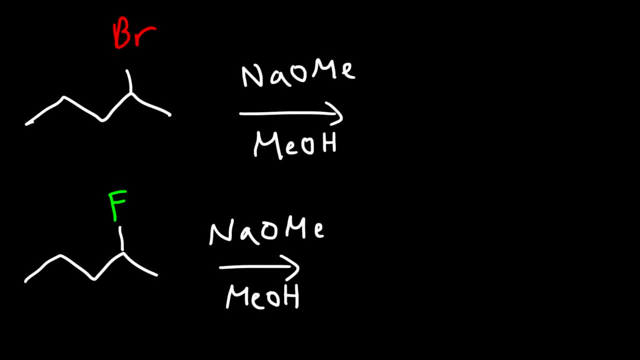 We have a strong base and a secondary alkyl halide. Strong bases favor E2 reactions over E1 reactions, And for an E2 reaction no rearrangements can occur. So therefore we could form the double bond only on the left side or on the right side. 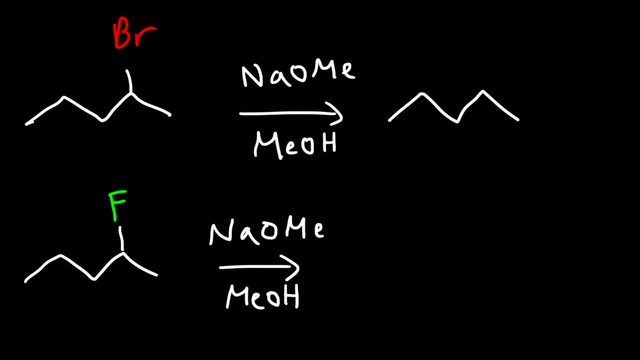 And using 2-brombopentane, the double bond will be formed on the left side. So that's going to be the major product And then this is the minor product, but we're not going to worry about that Now when using an alkyl fluoride. we're going 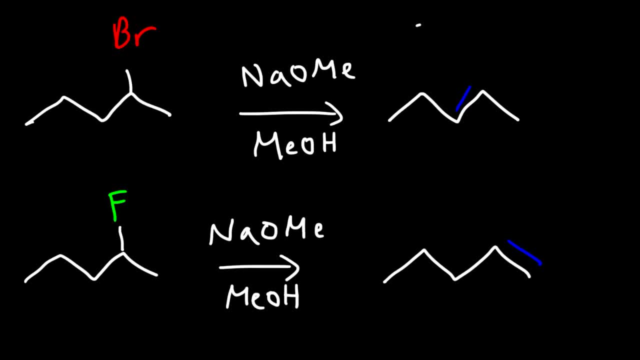 to get the Hoffman product as the major product, as opposed to the Zeta product. Now you might be wondering why. For one reason, the bromine atom is a good leaving group whereas the fluorine atom is a bad leaving group, And so bad leaving groups they tend to favor. 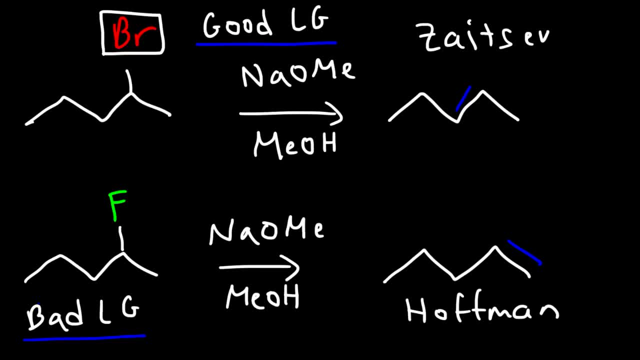 the formation of the Hoffman product, whereas a good leaving group tends to favor the formation of a Zeta product, Because bromine is a good leaving group. when this reaction occurs, the transition state will resemble more like an alkene than something else. 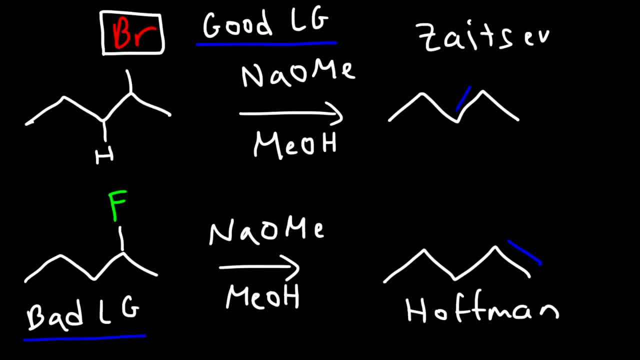 Because the transition state resembles an alkene. the most stable alkene is the one that's going to form And that's why we get the Zeta product. Now, when dealing with the bad leaving group, when the base comes in, to remove the hydrogen, this leaving group. 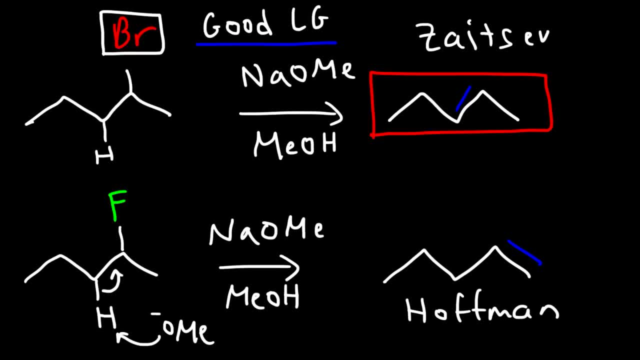 doesn't want to leave, And so it's pretty slow in leaving that substrate. As a result, there's going to be a buildup of hydrogen And so when the base comes in to remove the hydrogen, there's going to be a buildup of hydrogen, And so it's pretty slow in leaving. 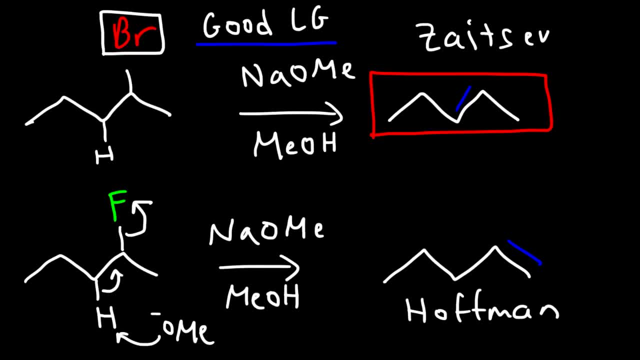 that substrate. As a result, there's going to be a buildup of hydrogen, And so the transition state resembles more like a carb anion rather than an alkene, And so we need to think of the stability of a carb anion For carbocations. we know that tertiary carbocations are more 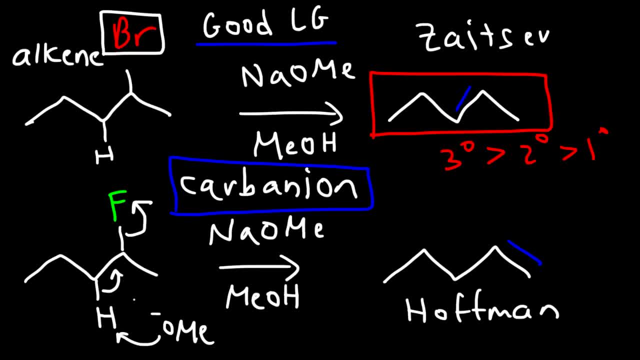 stable than secondary ones, and so forth, But for a carb anion, the reverse is true: Primary carb anions are more stable than secondary ones, which are more stable than tertiary carb anions. So therefore, the base wants to abstract this hydrogen better, because it will lead to a more 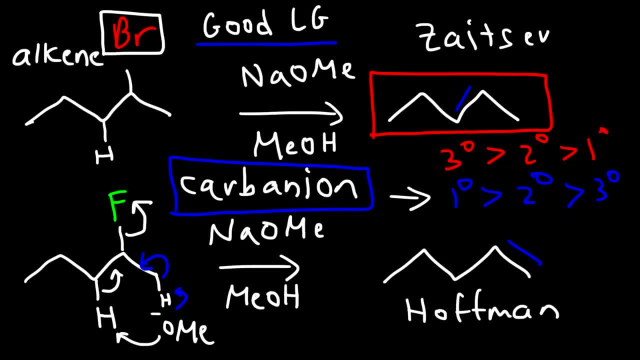 stable carb anion-like transition state. A primary carb anion is better than the tertiary one, So that's why it's better to form the double bond next to the primary carbon as opposed to the secondary carbon. So remember that. alkyl fluorides. 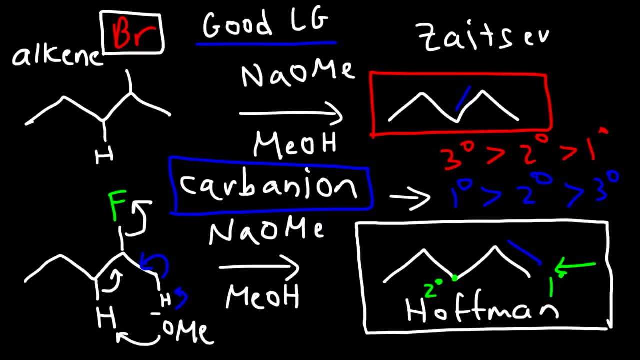 prefer to form the Hoffman elimination product, since fluorine is a poor leaving group and the transition state resembles more like a carb anion rather than an alkene, And primary carb anions are more stable than secondary or tertiary carb anions. Now, if you have a good leaving group like bromine, 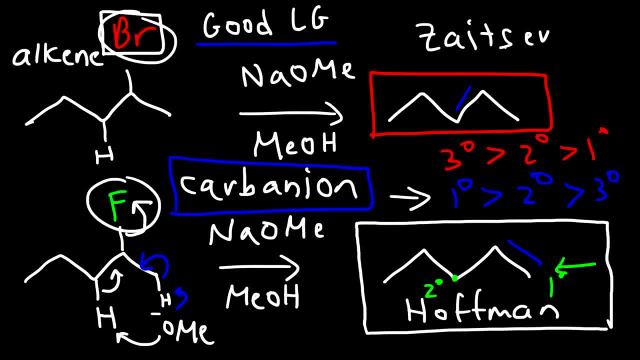 chlorine or iodine, then you're going to get the Zaitsev elimination product as the major product, since the transition state is more stable than the tertiary carbon. So that's why it's better to form the double bond next to the primary carb anions. That's why they're more stable than secondary. 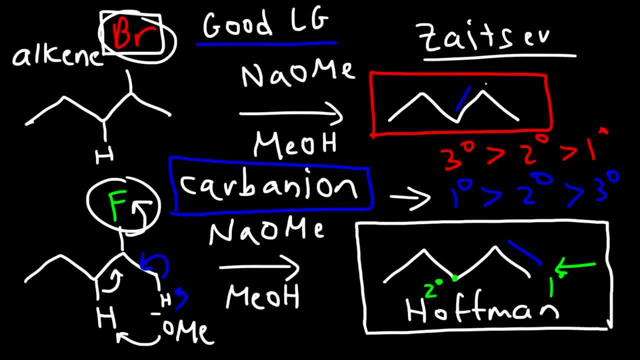 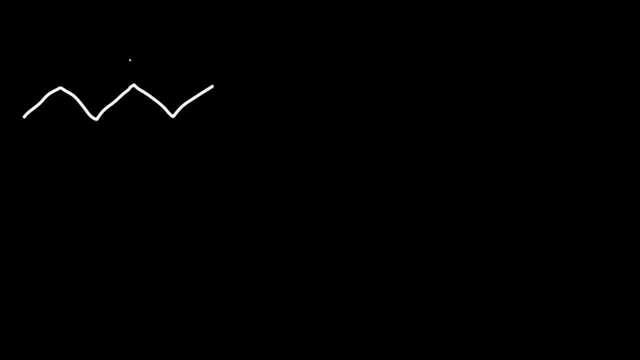 carb anions And that's what actually forms the Zaitsev elimination product. Whenever you terminate this type ofFk reagant, based on the amount of product that's in the pH, it canaffect more than atriple carb anions. but no matter the berry and valley. 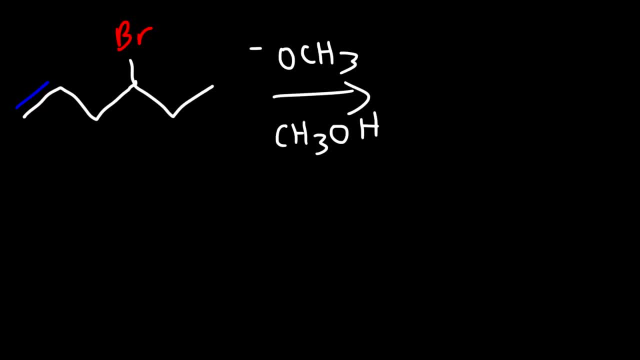 So that is full 인터�ケł, the E2 reaction for a secondary alkyl halide. Now there's two hydrogen atoms that we can remove: The blue hydrogen atom or the red hydrogen atom. So which one will the base go for? If methoxide goes for the blue hydrogen atom, the 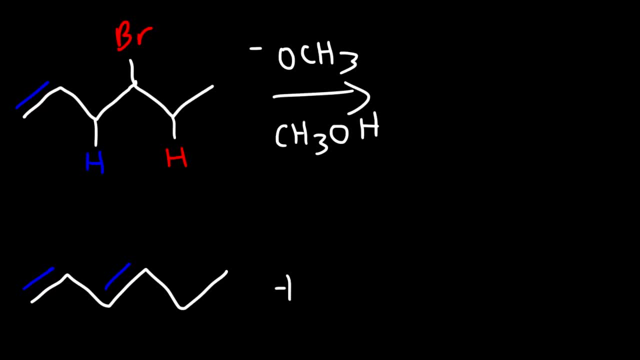 double bond will form on the left side of the bromine atom And if it goes for the red hydrogen atom, the double bond will form on the right side, And so this is an isolated diene. It's a diene because there are two double bonds And 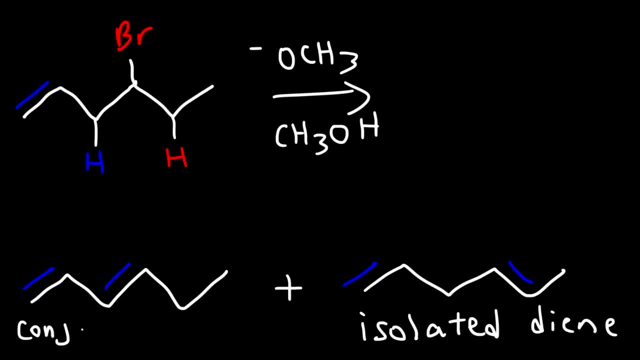 on the left, we have a conjugated diene. You need to know that conjugated dienes are more stable than isolated dienes due to resonance. So anytime you have a double bond and a single bond and a double bond, you have a conjugated system. 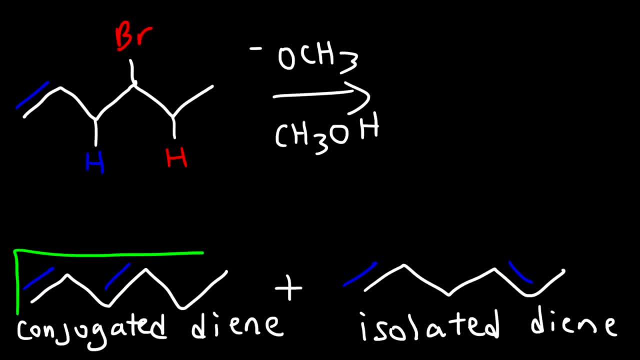 And so these alkenes are more stable. Therefore, this is going to be the major product. Okay, that is it. That's a terrible alkenes, Let's do that again. And here, this is the minor product. So, to draw the mechanism, the base is going to go for the hydrogen, The carbon.